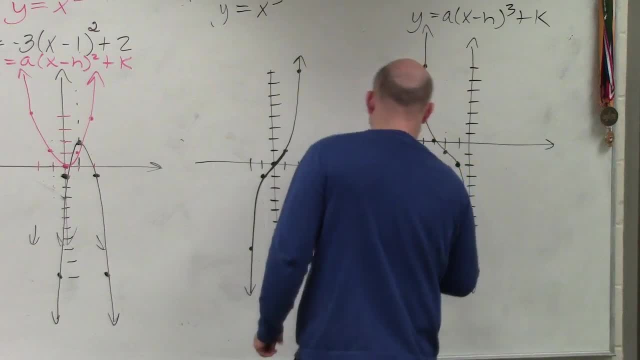 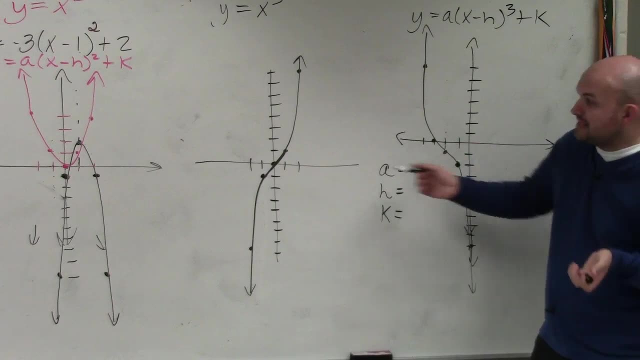 H and K. Okay, remember A: does your stretching or compressing? Does this look like it's been stretched or compressed at all? No, And the best way to kind of determine that is again look at the relationships. If you guys can see here this is over one up, one over one down. 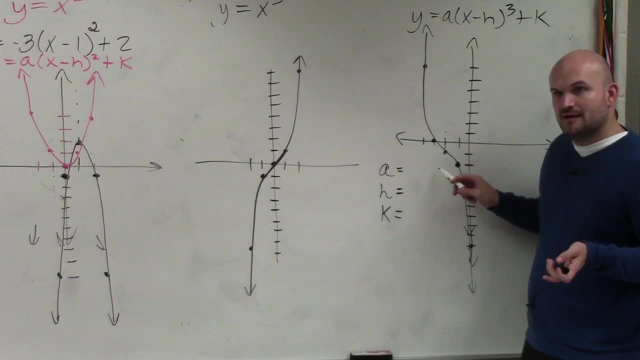 one. You guys can see that this relationship is kind of the same right. But if it was like over one up three, right, You could say that, oh, it's been stretched right, So therefore A would have to be a larger number, And if it was like over one up one third, it kind of been compressed. 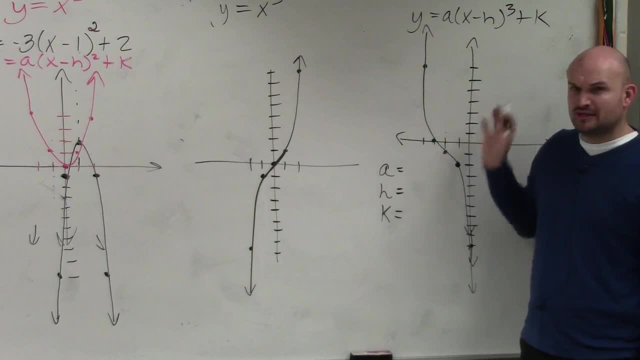 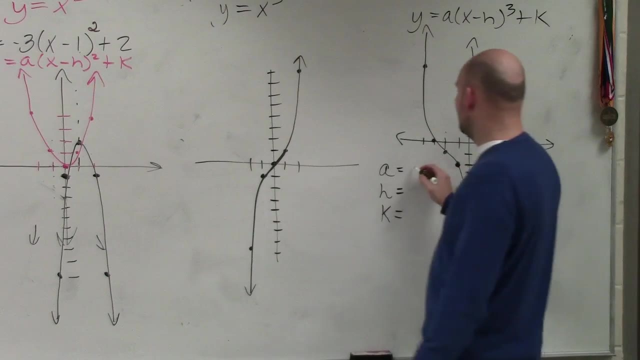 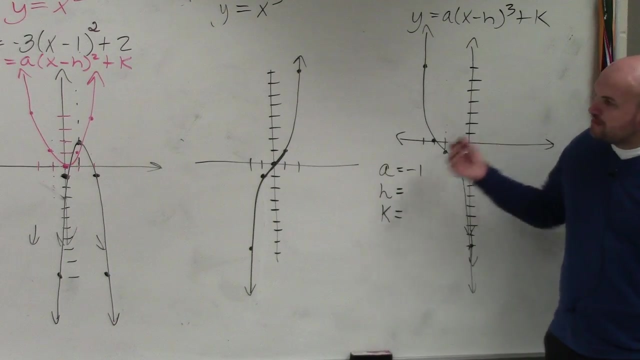 right, But it looks like that's about the same. However, they don't look like the same shape. They kind of look like one has been re-lected over the X axis. So A I'm going to call as a negative one, H represents your shifting left to right. So the focus point for a absolute value. 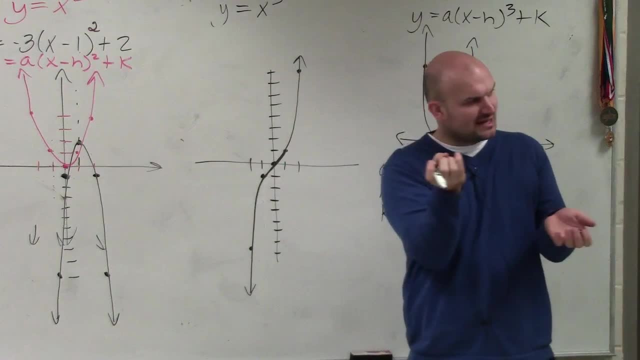 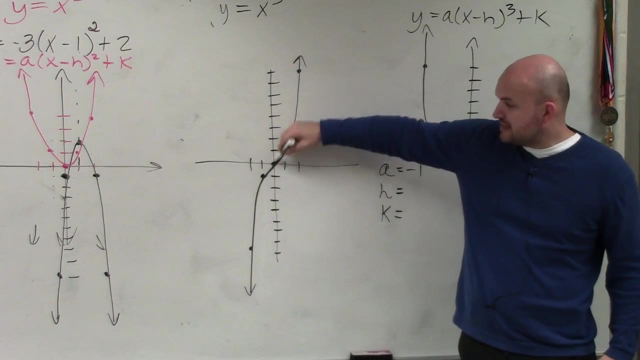 and a parabola was pretty simple. It was always that turning point, the vertex, right. Well, this one doesn't really have a vertex. It does have a turning point, though, So what I like to do is I always like to create this double turning point here as kind of like my 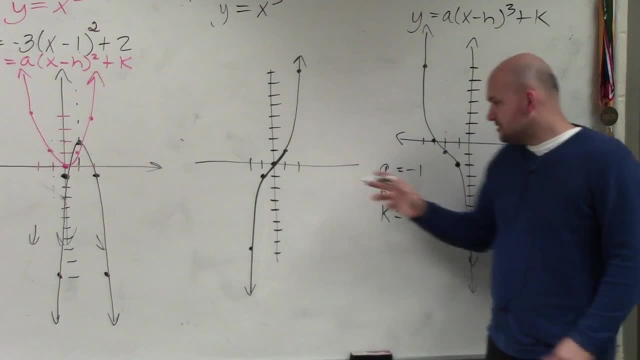 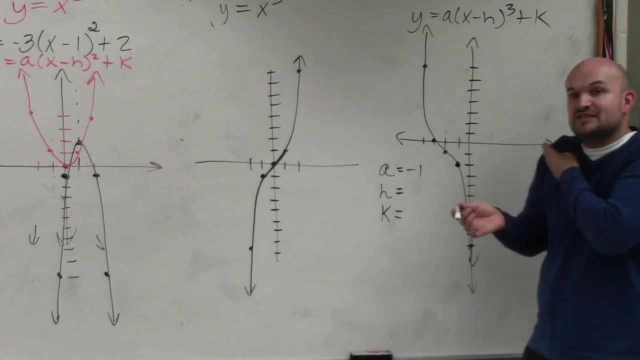 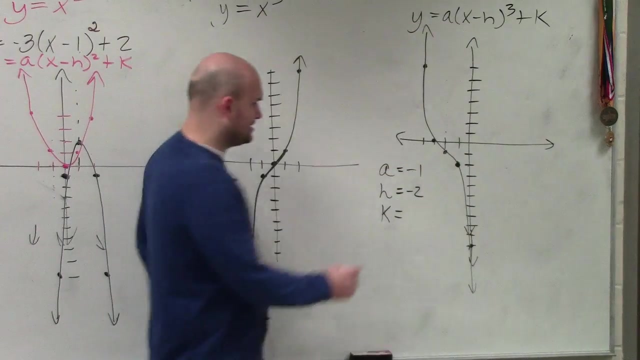 focus point That's at the origin, That's my focus point. So you can see that focus point has been shifted left to down one right. So how do I represent shifting to the left two? Well, that means H is going to be negative and K down one is going to be a negative one. So if you were to plug 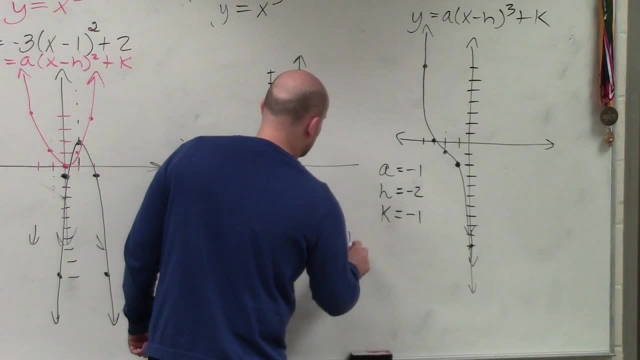 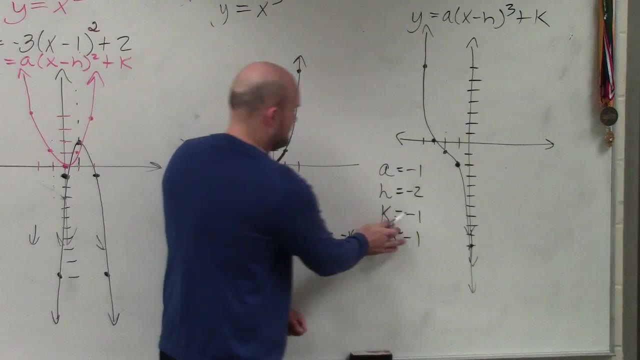 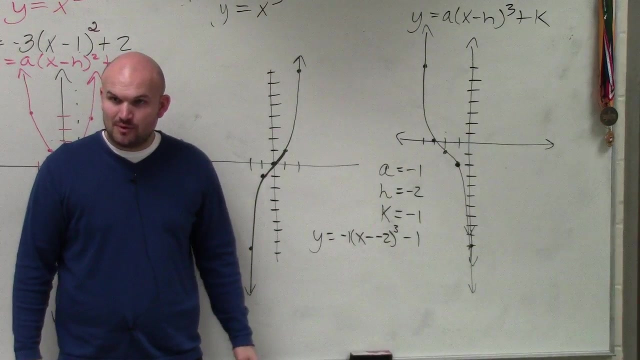 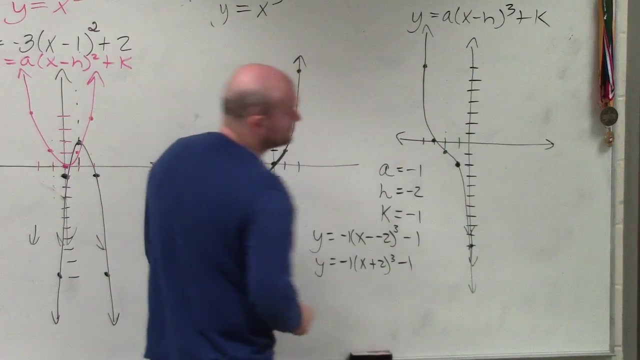 these into the equation. it would look like this: Y equals negative one, X minus negative two squared minus one, Cubed, Thank you. Hold on. X minus a negative two is what X plus two. Okay, Does that kind of understand why it's like that opposite thing? Yes, 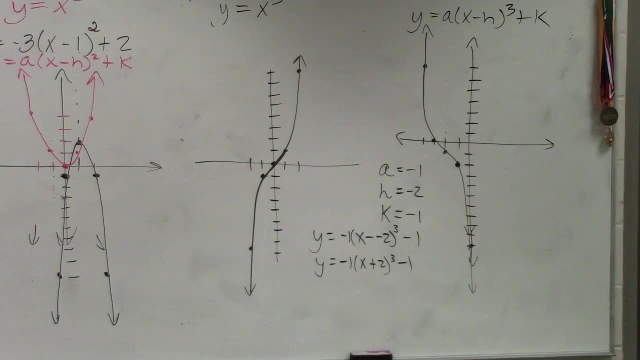 All right, One last thing to go over real quick. 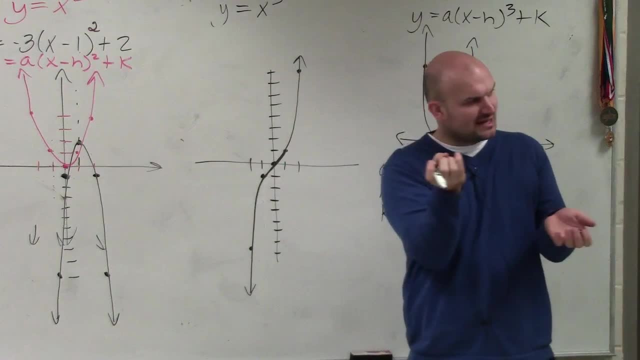 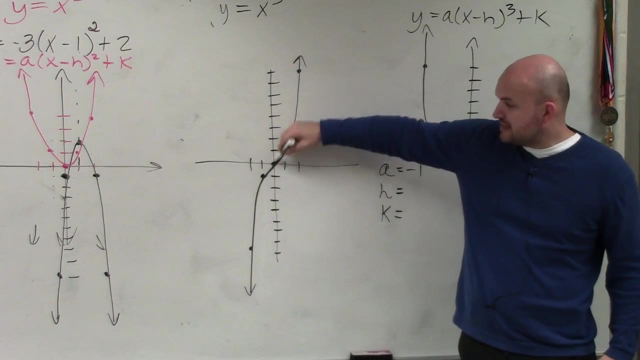 and a parabola was pretty simple. It was always that turning point, the vertex, right. Well, this one doesn't really have a vertex. It does have a turning point, though, So what I like to do is I always like to create this double turning point here as kind of like my 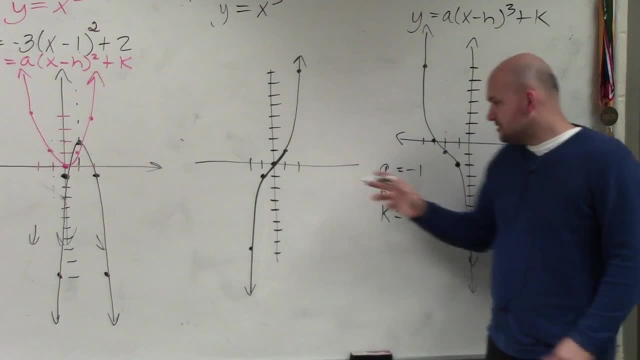 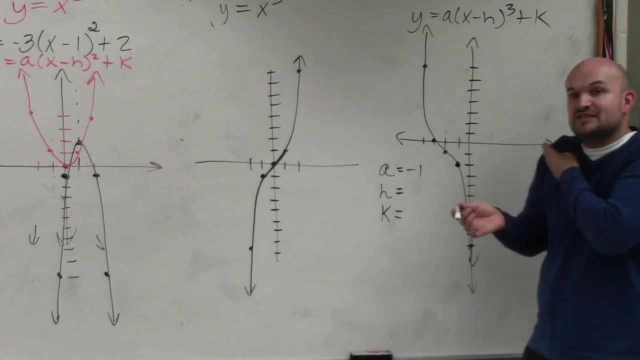 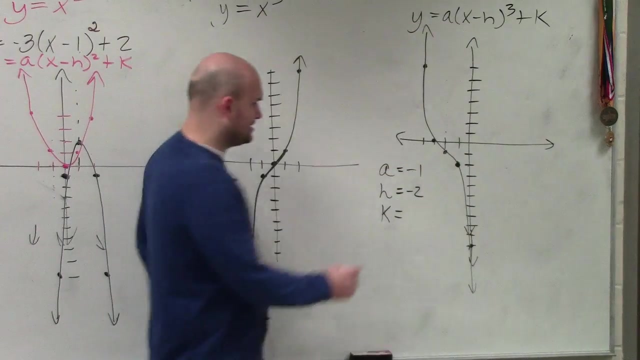 focus point That's at the origin, That's my focus point. So you can see that focus point has been shifted left to down one right. So how do I represent shifting to the left two? Well, that means H is going to be negative and K down one is going to be a negative one. So if you were to plug 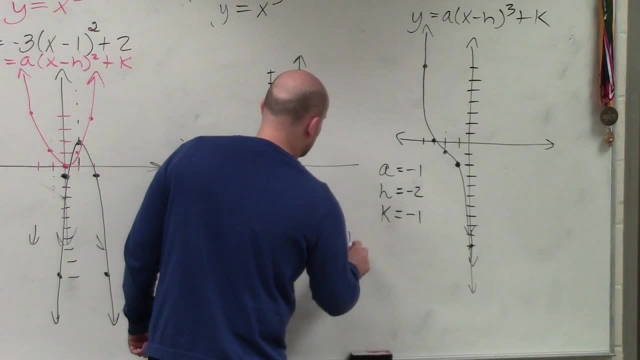 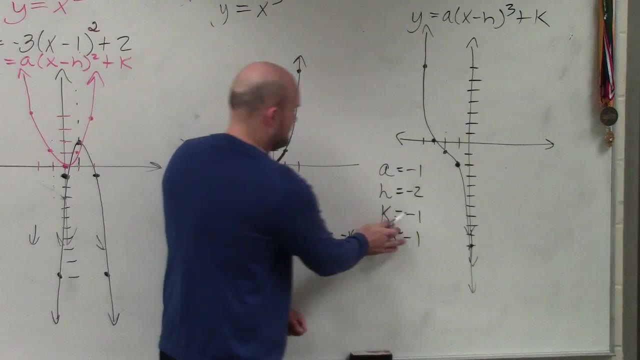 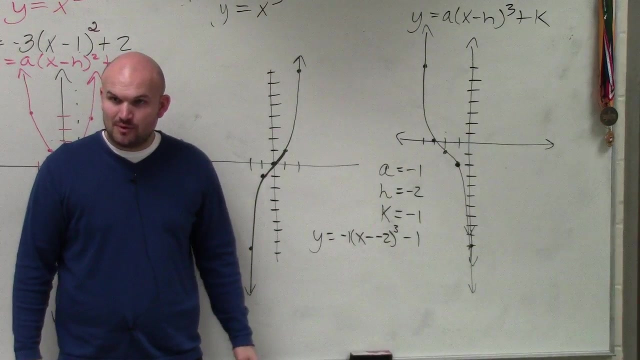 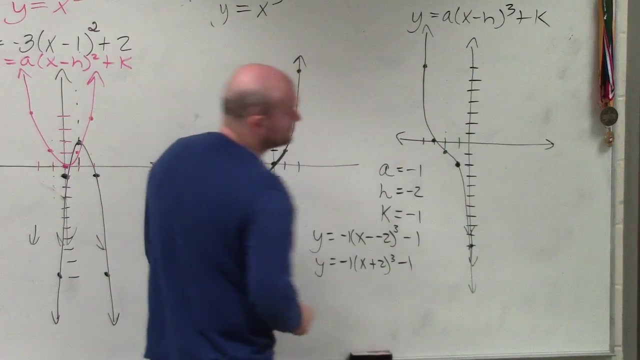 these into the equation. it would look like this: Y equals negative one, X minus negative two squared minus one, Cubed, Thank you. Hold on. X minus a negative two is what X plus two. Okay, Does that kind of understand why it's like that opposite thing? Yes, 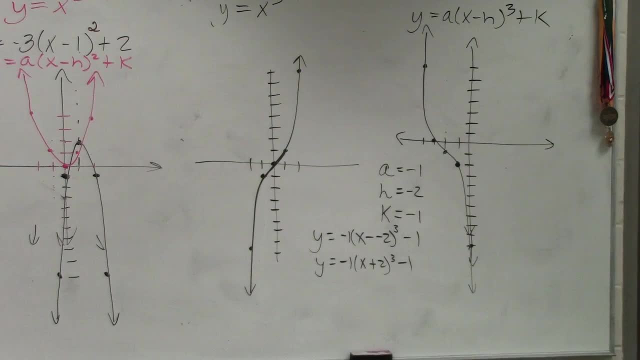 All right, One last thing to go over real quick. 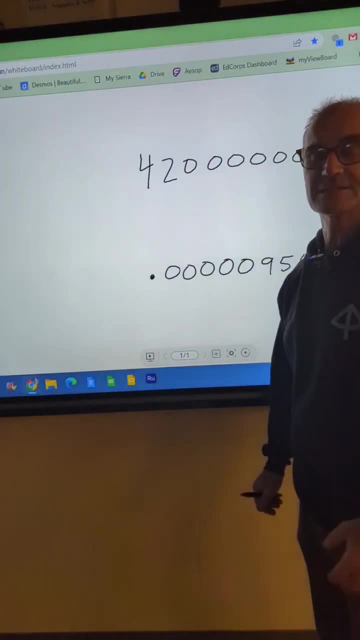 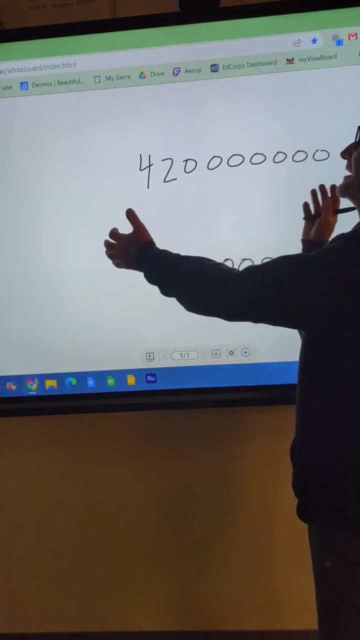 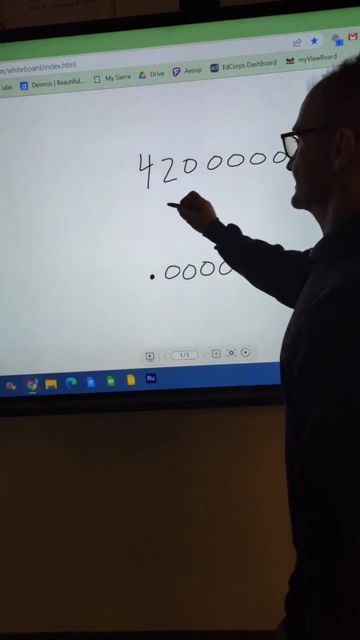 All right, quick video on how to put numbers in a scientific notation. Scientific notation is a number between 1 and 10 times 10 to a certain power. It allows you not to have to write out these really big numbers like that. So if I want to put this 420 million in the scientific notation, 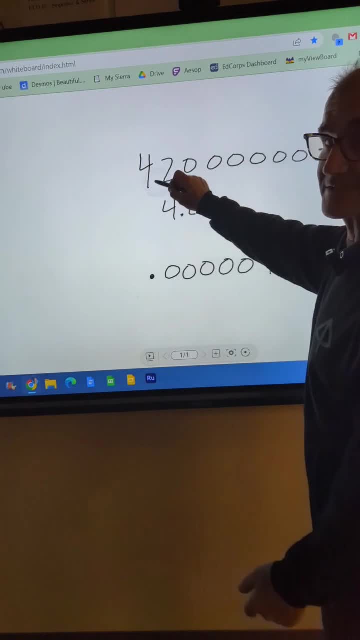 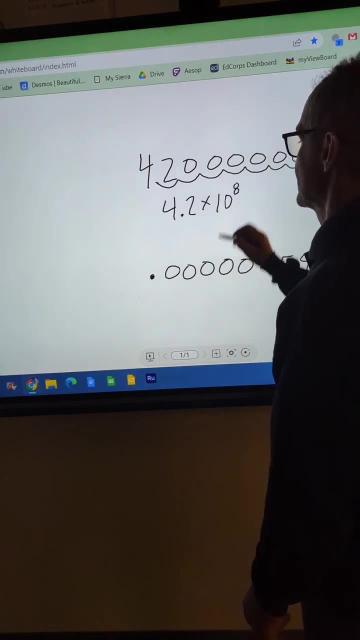 it's going to be 4.2.. I'm going to count up how many places that decimal went over: 1,, 2,, 3,, 4,, 5, 6,, 7,, 8 times 10 to the 8.. If I got a really small number like this, I could put it in a: 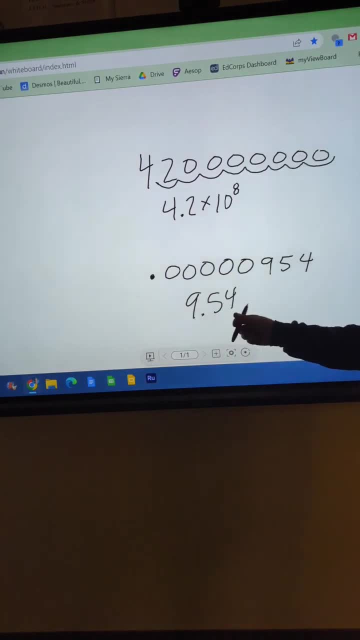 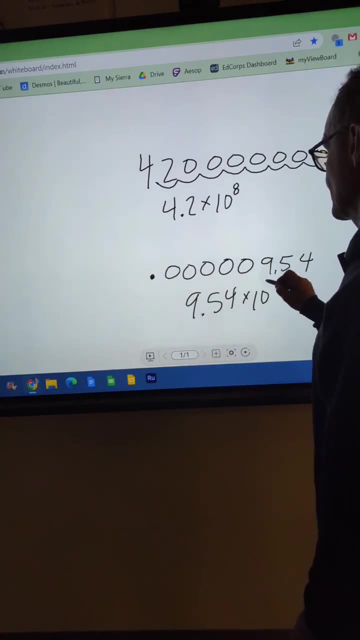 scientific notation. Again, this number is between 1 and 10 times 10 to the number that the decimal place goes back over here. So it's going to go over 1, 2, 3,, 4, 5, 6.. It's going to the left. 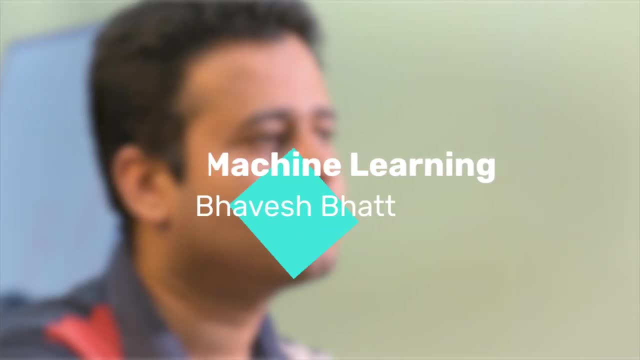 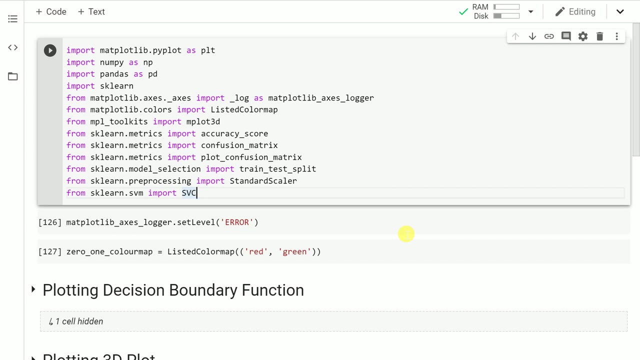 We all know the power of support vector machine. In this video I'll explain how sometimes, when your data is not linearly separable, support vector machine fails to give you the accurate model. What do we do in that case? We utilize something called as a kernel trick.